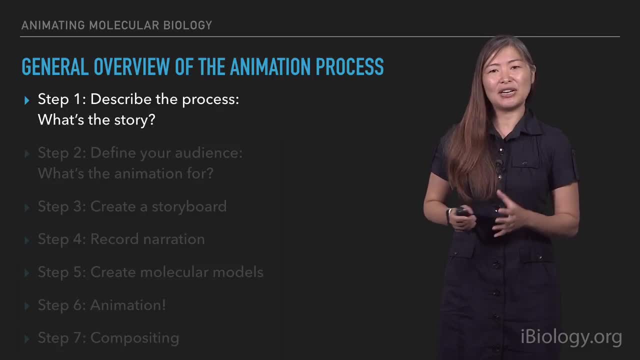 In animation. you really have to do this in much more detail than you would if you were just drawing a figure. So, but you need to ask the question of you: know what's happening? Where is it in the cell? How many proteins are there? 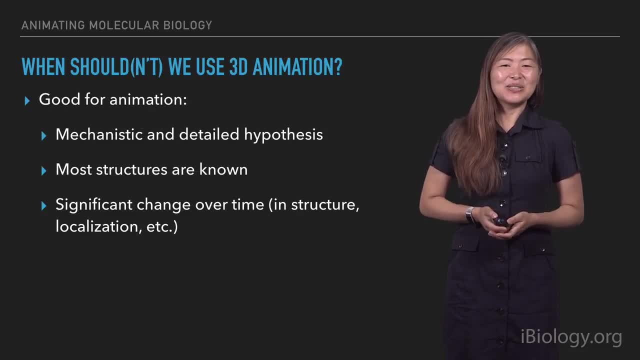 And, in particular, what structures or other data may be available to tell that story. So one thing to note is that not all processes are great for 3D animation. So in general, the things that you think about that are really good for animation. 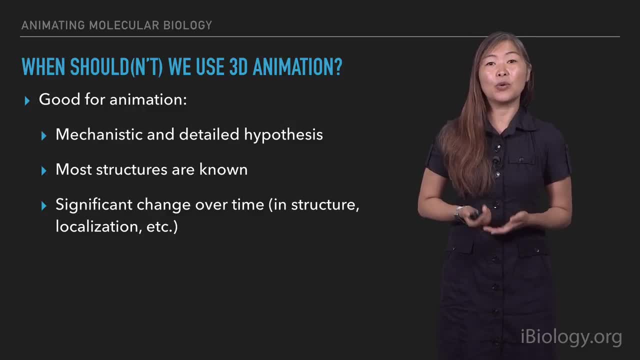 are processes where we really have a very deep mechanistic understanding of what might be happening, or at least an idea that we want to put forward. that's very, very detailed. It's also great when we have most of the structures are available so that we can use those directly into the animation. 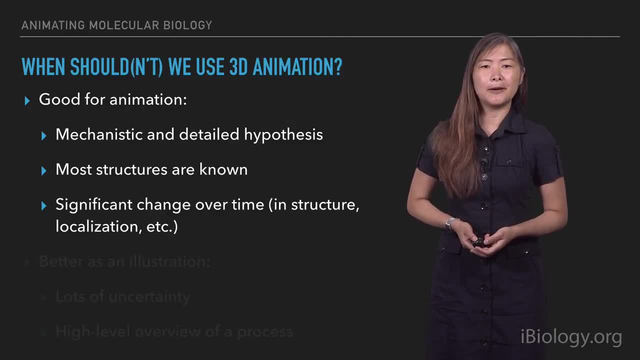 And we're also showing something that changes significantly over time. Some of the things that may be less great for 3D molecular animations are processes where there's a lot of uncertainty, where we're not quite sure what's happening at different, at multiple different stages of the process. 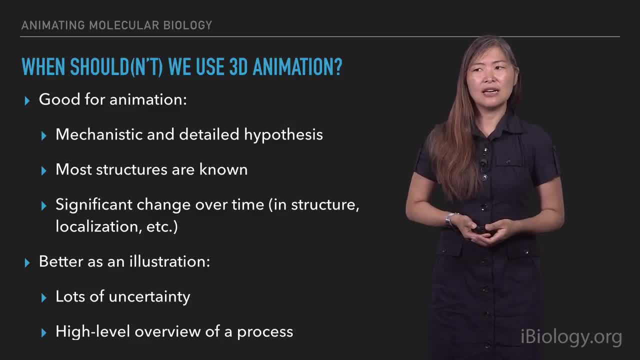 And also where we're providing maybe a high-level overview of a process, because the nature of the molecular animation- a 3D molecular animation- is to show a great amount of detail, So it's kind of harder to show a general overview. 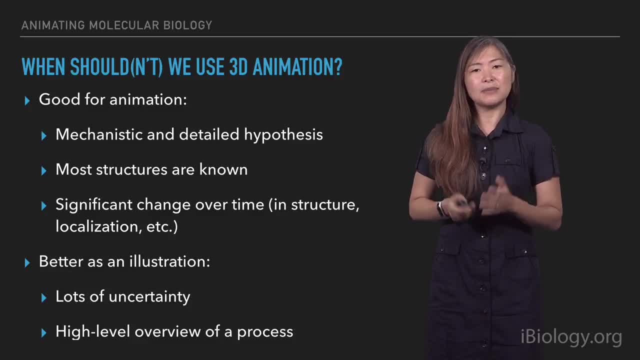 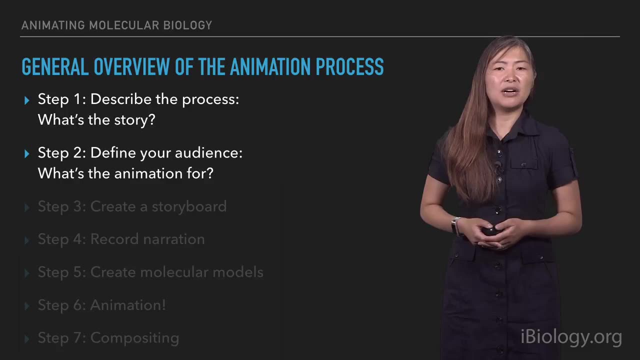 when we're really kind of digging pretty deep like that, And so for those types of processes, it might be better to consider creating a 2D illustration or even a 2D animation for those processes. Alright, So once you've described that story, 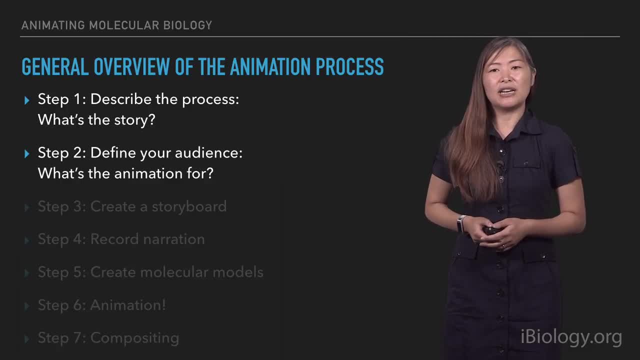 next you, you have to think about your audience. Who is this animation for? In general, when I work with other people, with my collaborators, there are two major types of animations that we create in sort of the research sphere. One is animations that are created. 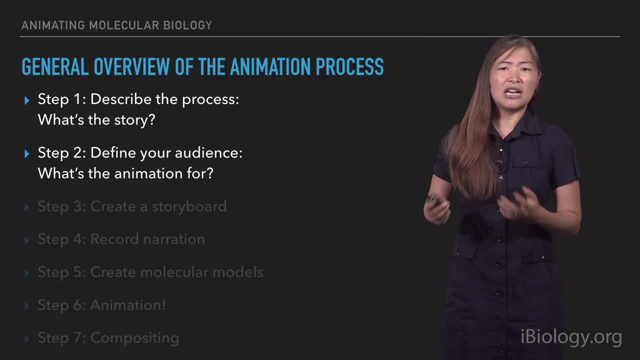 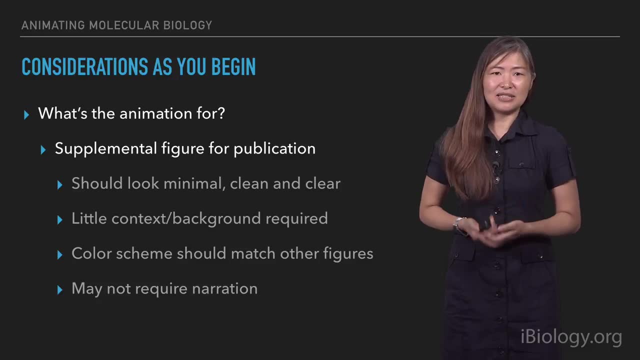 for supplemental figures. And the second is animations that are made for a kind of a more general audience, for use both in talks and in real life. So when you're thinking about an animation for a supplemental figure you may have different considerations than kind of a broader audience. 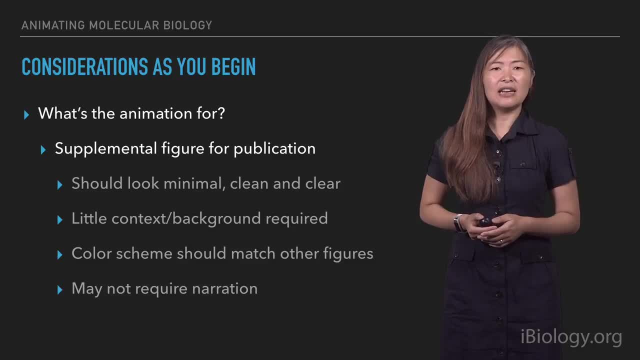 So in supplemental figures you usually have a pretty targeted audience that has probably a good knowledge of the background that's needed to understand that figure. So as a result, and you want to really convey ideas as quickly and efficiently as possible, So in general for supplemental figures, 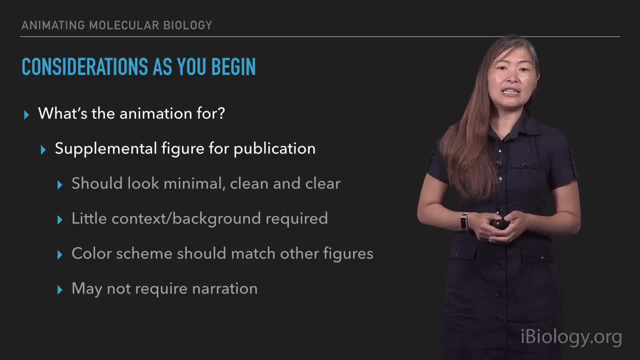 not a lot of background, not a lot of context is generally needed. Another thing to think about is that the color scheme that you use in these animations should match the other figures. So if you have a figure 2 somewhere that shows like a model figure, 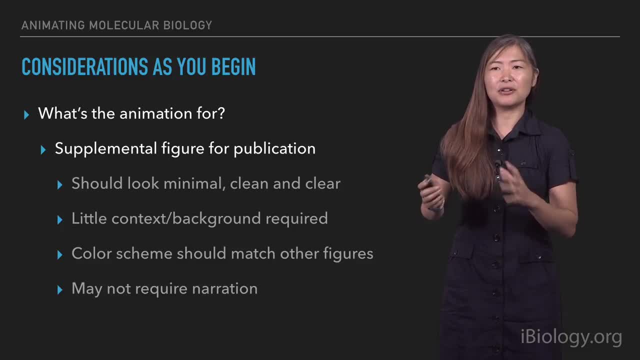 the animation should really match. It should be the same color scheme And other kind of elements should be really passed from a figure or a description in the paper to that animation. So supplemental animations, figures for animation, animations used as supplemental figures may or may not require narration. 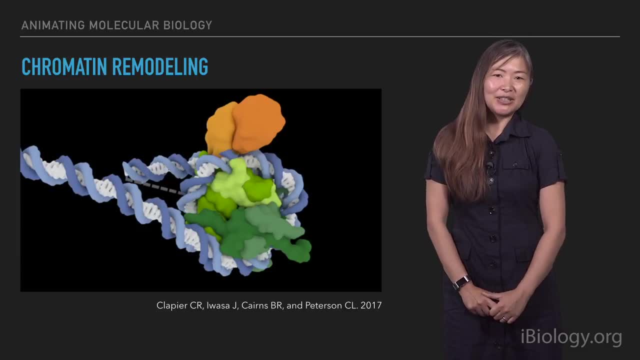 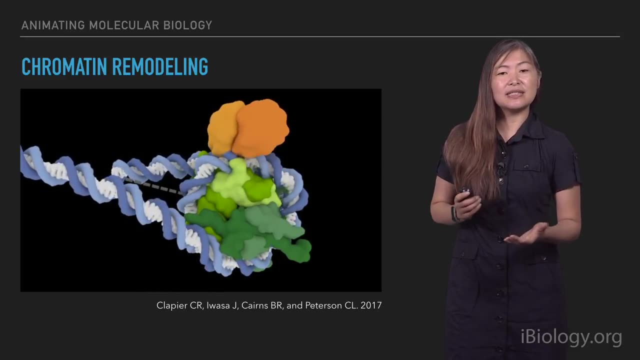 So this is an example of an animation that was created for a supplemental figure. This was made for a review on chromatin remodeling, And what we have is this animation where, again, I've used the same kind of color scheme that's used in the rest of the paper. 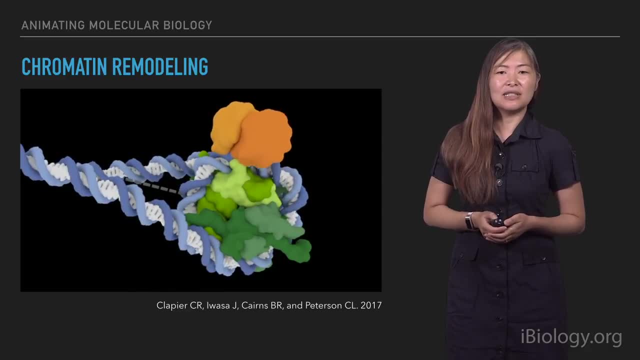 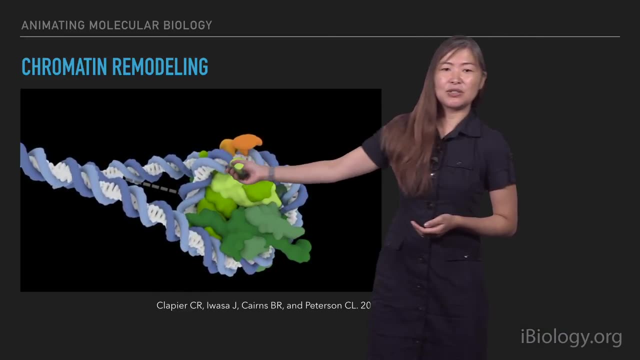 So really the viewer can look at those figures and then watch the animation, and everything is relatively seamless. So this is kind of some of the visual representations that were used in other parts of the figure. for example, we had this gray axis. 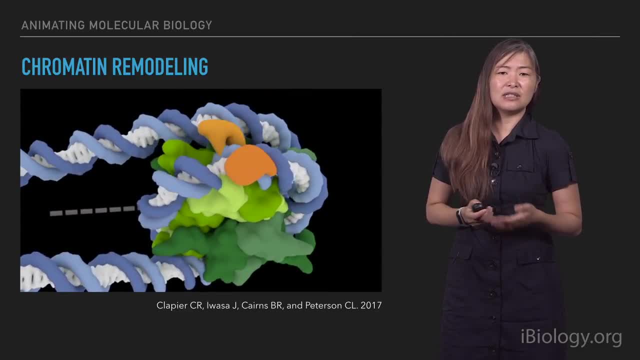 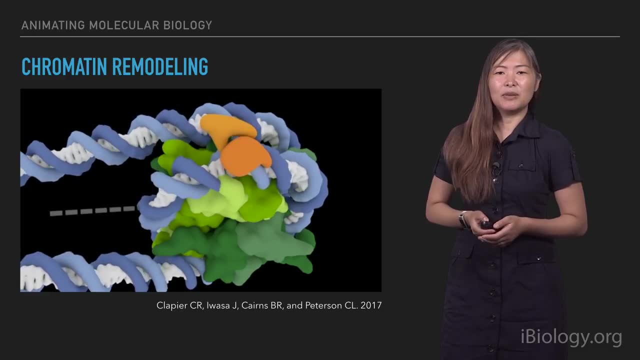 that marks the central point of this nucleosome And so that's used in other parts of the of figures in the review as well. So these are all things to consider, And again, here the background is pretty minimal, There's not a lot of storytelling. 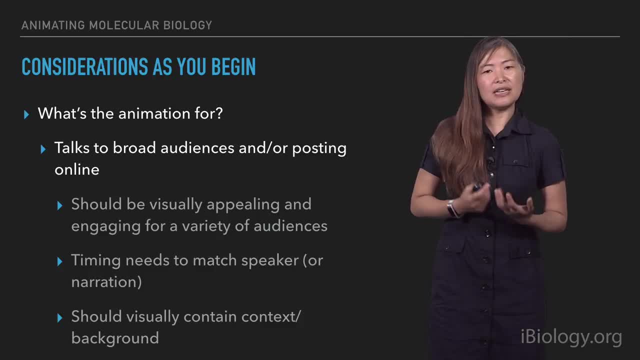 that's going on behind the scenes there. So when you're thinking about an animation that's really for broader audiences, this may be both either for a talk or for posting online. different considerations have to play a role here. So one of the things you have to think about: 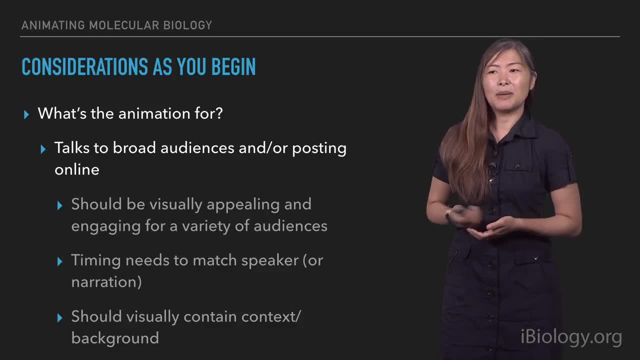 is that audience? So if you're trying to appeal to a high school student, a member of the general public, you really need to tell a story well, in an engaging way, And so this usually means that you have to try to make it as visually appealing as possible. 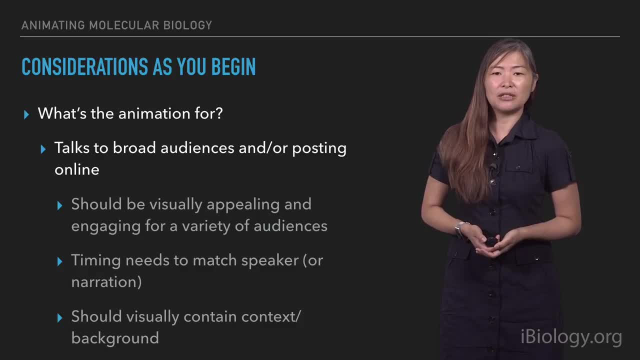 Adding context and background will really help people understand the story better, And oftentimes these are going to be narrated animations, So timing needs to match the speaker's narration. So an example of this type of animation is shown in here. 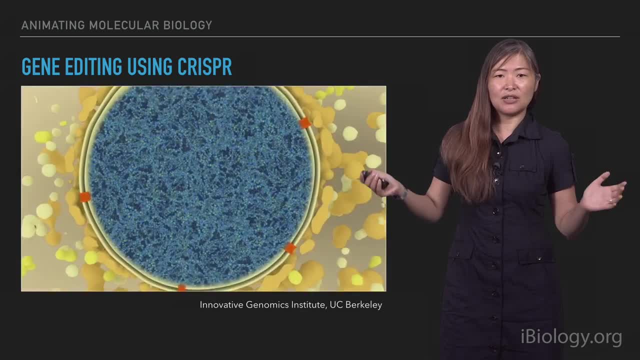 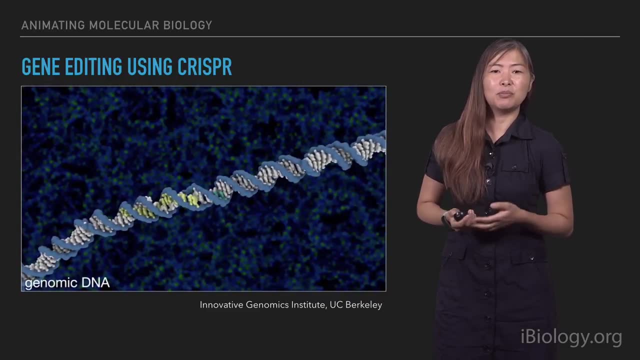 So this is an animation of gene editing using CRISPR And what you can notice. we started with an entire cell. We're zooming into the nucleus, We're seeing all this kind of chromatin in the background. to give a little bit more of that story, 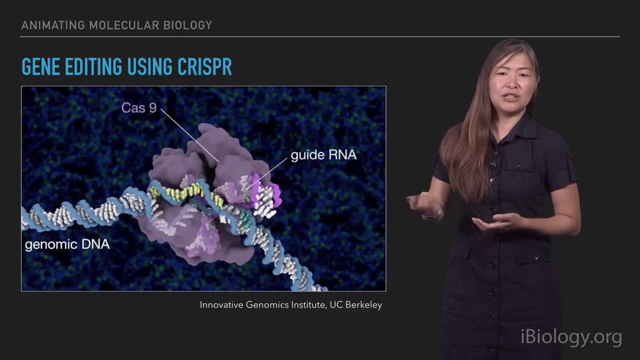 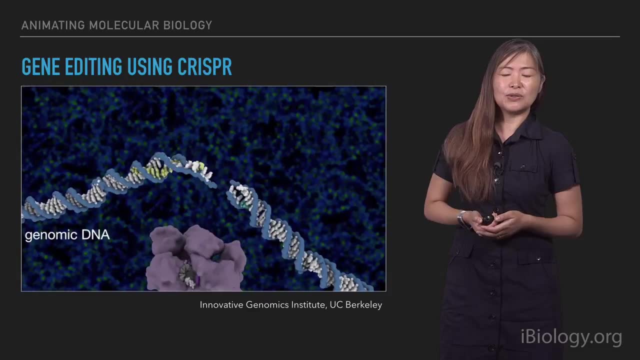 And there's also a lot of labeling here to make sure that the viewer is able to really follow what's happening. So we're going to start with that DNA and then cutting it, And then a new piece of DNA is being introduced, And so the labeling helps. 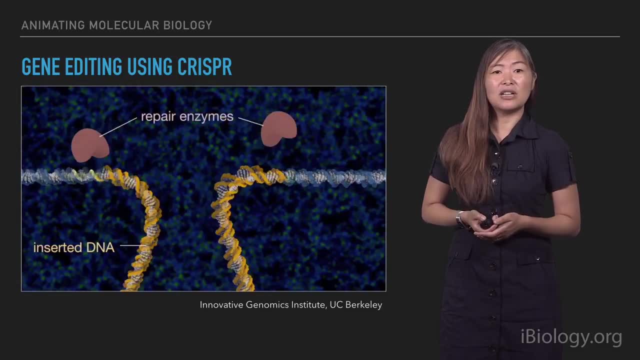 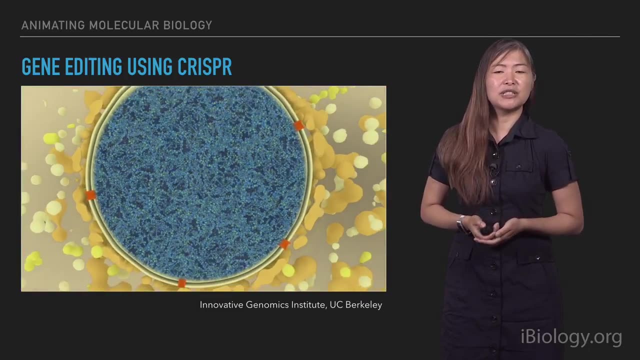 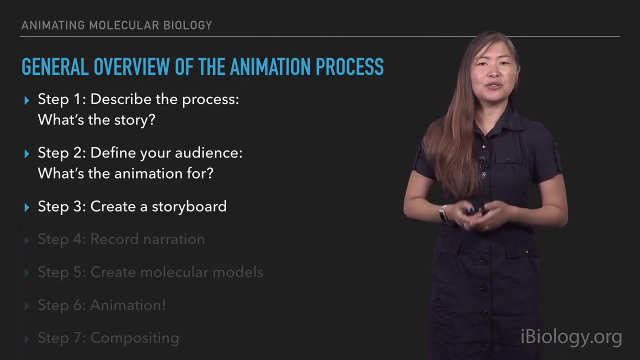 This animation also typically is run with narration as well as with music, And so that really helps, I think, convey make the animation a little bit more memorable for different viewers. So next, once you've kind of gone through the process of thinking about your story, 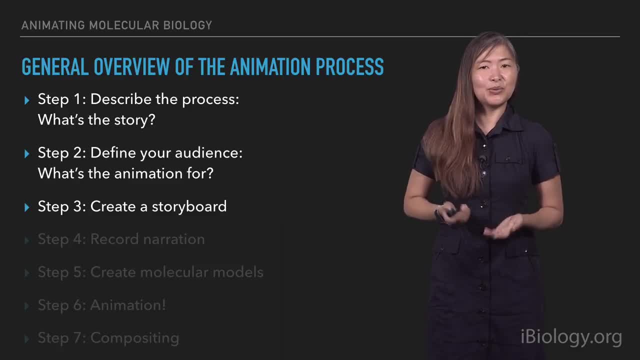 what is it going to tell? and, thinking about your audience, how do you create a storyboard? And a storyboard is similar to probably what you've heard that animation studios do, but on a much, much smaller scale. So storyboards is really. 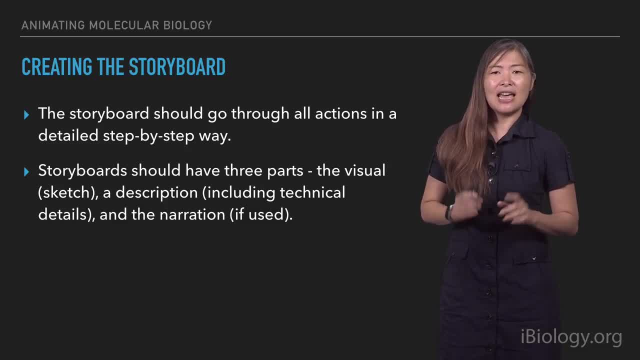 it's kind of a way of drawing out what happens at each step of the animations, And the ideal storyboard should really walk through every single step. Every single major change in the animation should be drawn out in the storyboards In general, the storyboards I create. 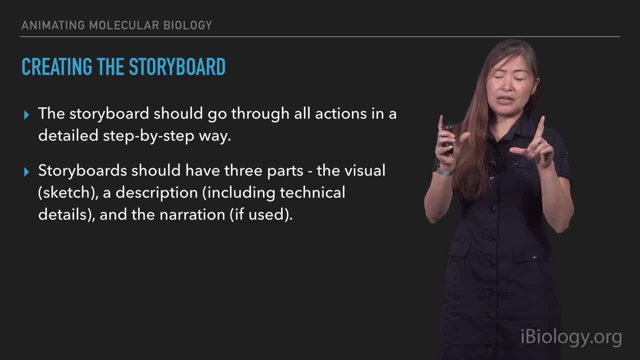 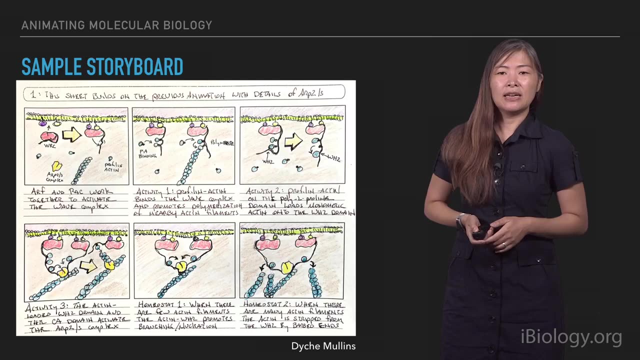 have three parts, two to three parts. So one is a simple sketch of what's going on, The second is a description, just written in text, of what's happening And then usually, depending on whether the animation has narration, 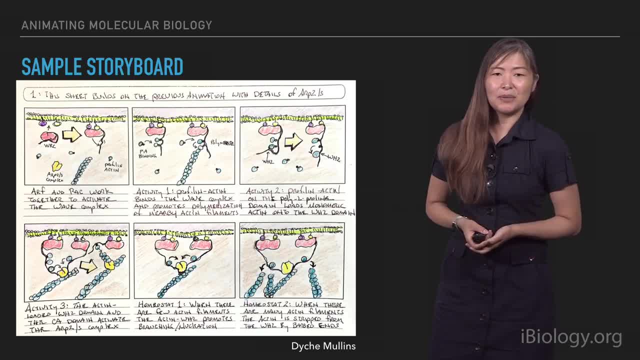 it'll have that narration as well. So a three-part. So this is an example of a storyboard. This was drawn by Dyke Mullins on a collaborative animation that we're working on, So you can see here he's drawn in kind of a comic book style. 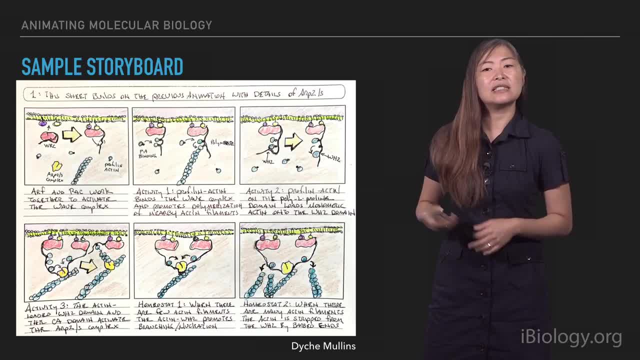 that kind of steps time in time as well as movement. He's done a lot of labeling and he's also written this description, So you know you can. I've made this kind of a template to be able to draw these storyboards. 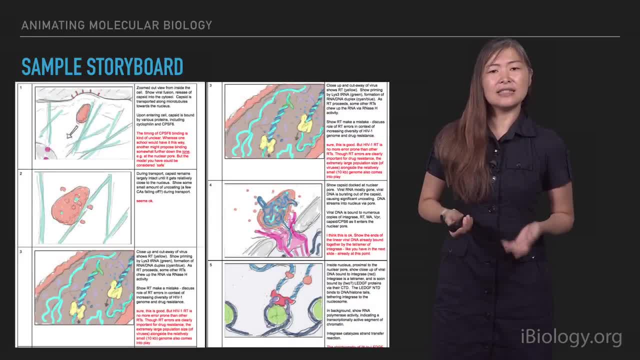 and you can create these pretty easily yourself or download them online for free. This is another example of a storyboard. So many of my storyboards are collaborative, The animation projects are collaborative And you know one of the major points of doing a storyboard. 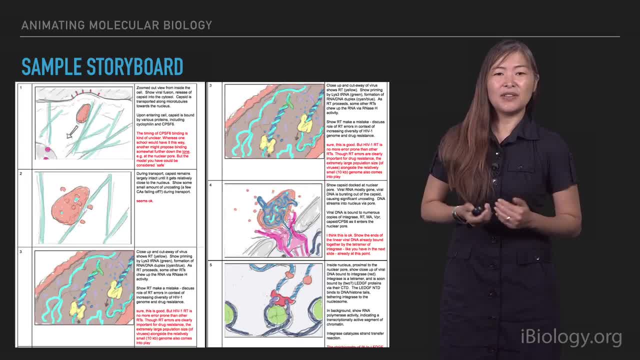 is really to save time on the animation process By defining every step of the animation, by showing that to your collaborators, with your team members, you're hoping to really minimize the amount of changes you have to make once you're in the animation software. 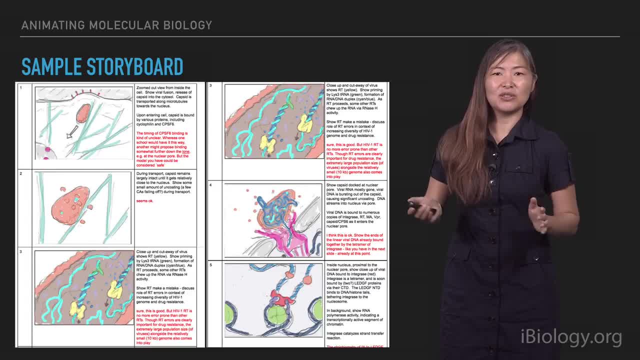 because that can get super time-consuming And so you're trying to address all of the problems kind of as early as you can, And so in this particular storyboard which covers the integration step of HIV infection, I've shared this storyboard which I've created. 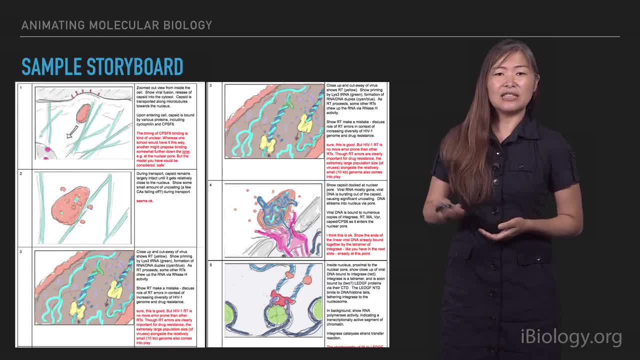 with a collaborator who's an expert in the field, And so he went ahead and made notes in red about things that he would change or alter in the storyboard, And so I can go back and change that before I go into the animation software. 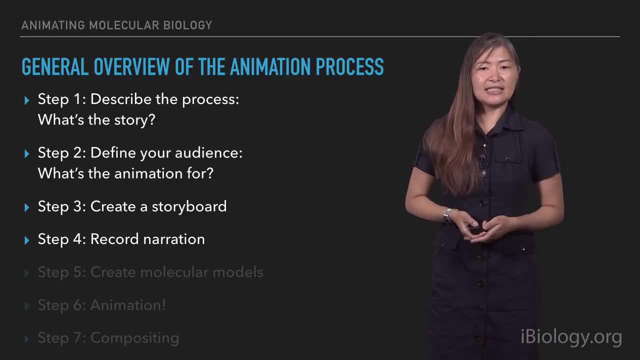 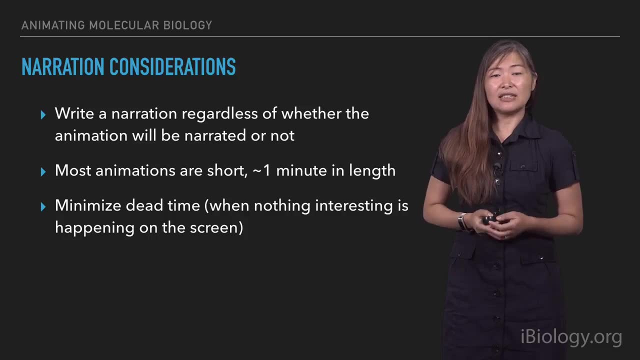 So it's really about saving time and being efficient. So next, after you create the storyboard, the next step is to record a narration. My general recommendation is to write a narration and record it, no matter whether you're planning on using a narration in your animation or not. 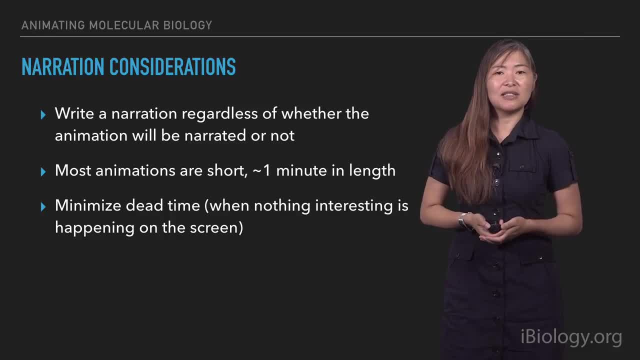 And this is because when a narration will get used in a talk or something like that, it needs to match the timing of the speaker. You need to know whether you know. basically, a long time is going to be spent on this part, describing this process. 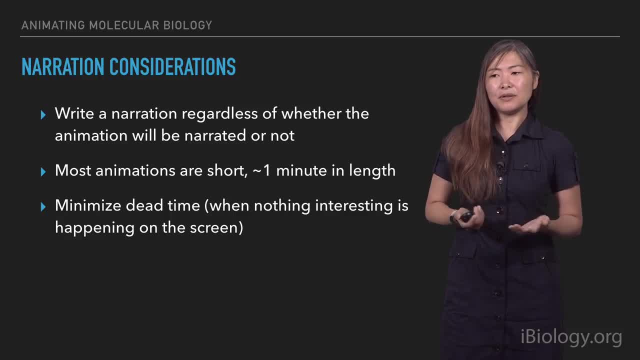 so that the animation- you know basically what the timing is going to be. Another thing to keep in mind is that animations are short. They're typically especially molecular animations. they typically are less than a minute in length, and so you have to be pretty concise. 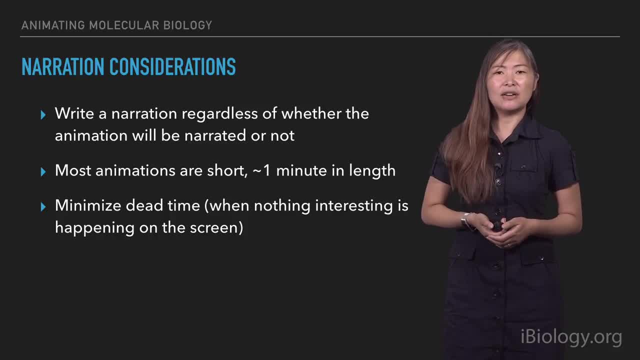 You have to be able to define the narration. Often you can do that outside of the context of the narration of the animation. And you also want to minimize dead time. You want to minimize time where you have some narration that's going and nothing is happening on the screen. 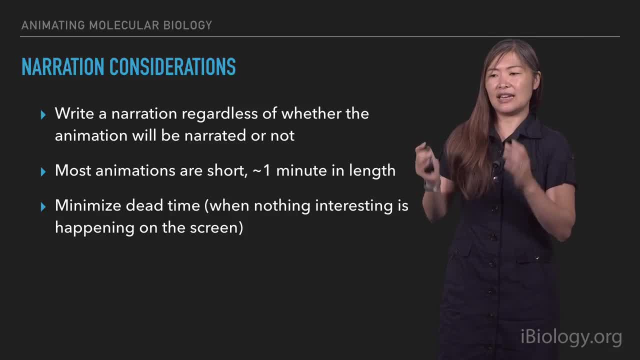 So it's really a good idea to try and really define the narration and the animation hand in hand. So writing out a narration and recording it is pretty much should be a very, very early step once you go into the animation software. 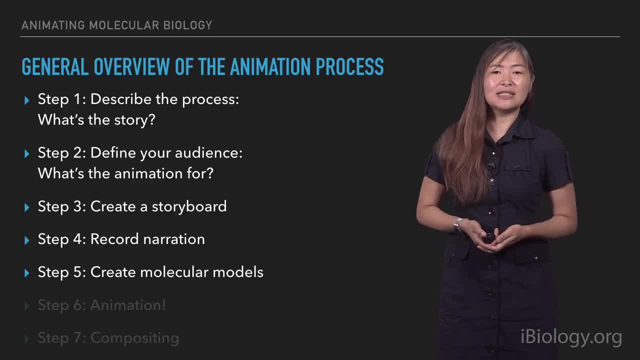 The next step is creating the molecular models. There are a couple of different major softwares that allow you to basically export a molecular model from, for example, a PDB and import them into various 3D animation software. So my favorite software to use. 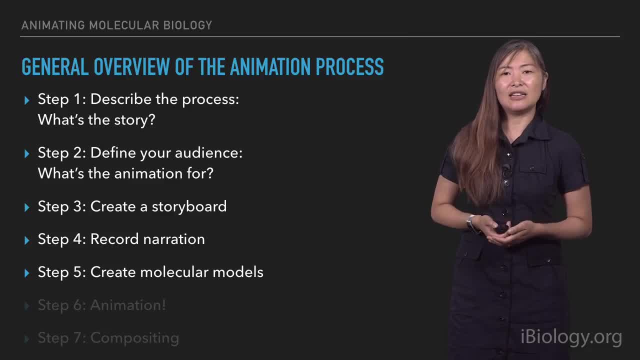 the one I'm most familiar with is UCSF Chimera. That's free and free to download, And a lot of other people also can use PyMOL. That can be used to also generate 3D models. So I'll be talking you through. 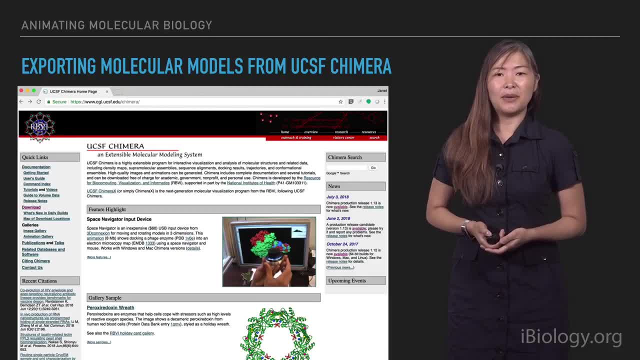 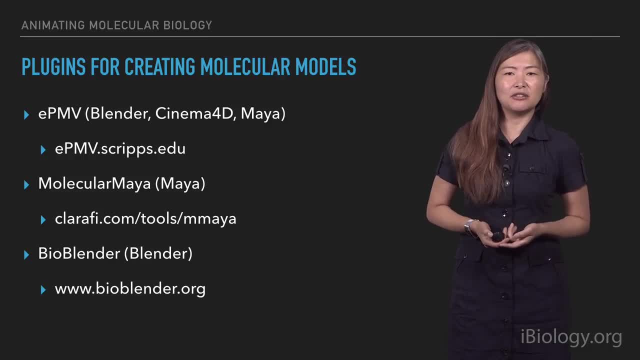 my process of exporting molecular models from UCSF Chimera in just a couple of slides. Another thing to note is that you can also import molecular models using a number of different plug-ins for different 3D software. So I'll be talking in the next video. 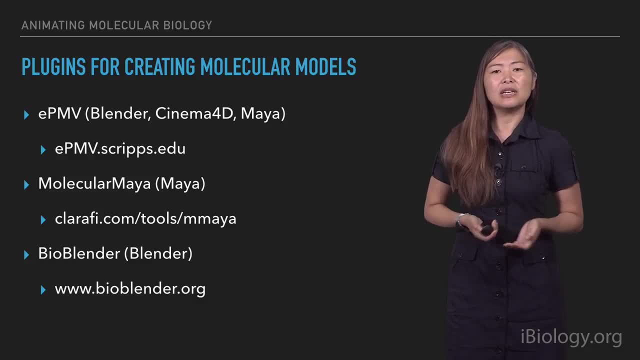 about really the animation process and different software you can use, But I'm just noting here that you can import PDBs using a number of these different plug-ins, including ePMB, and these are for specifically for some specific types of 3D animation software. 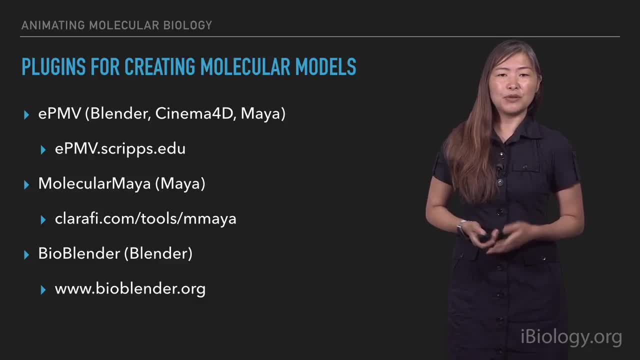 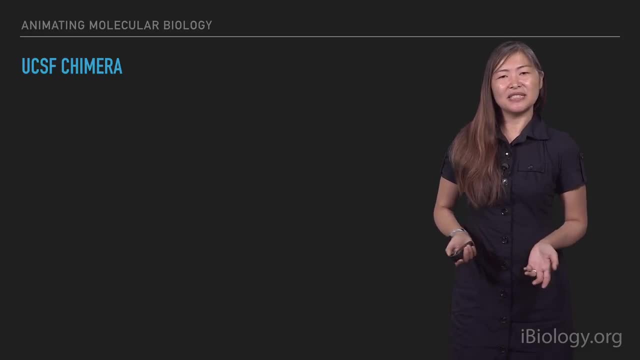 There's also molecular Maya and BioBlender. So those are things that are worth looking into. if you're using these specific software and you want kind of a shortcut to importing PDBs, Alright, so let's jump into Chimera and I'll show you the process. 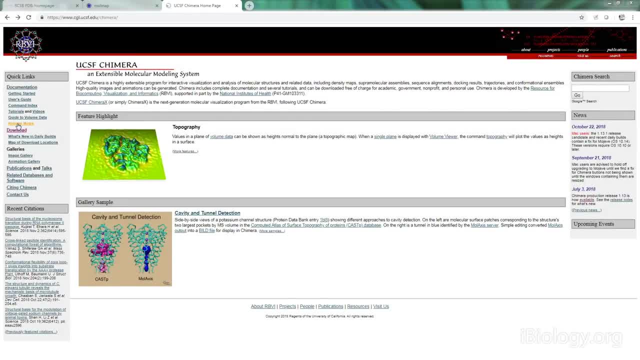 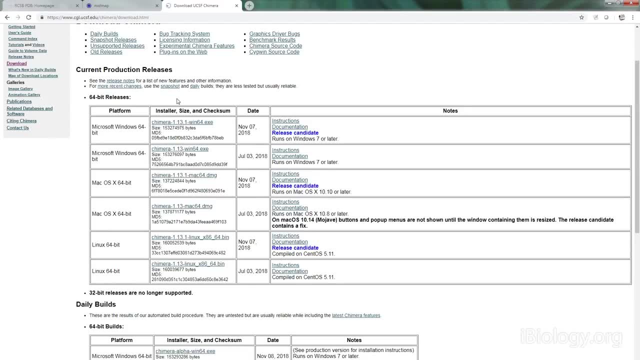 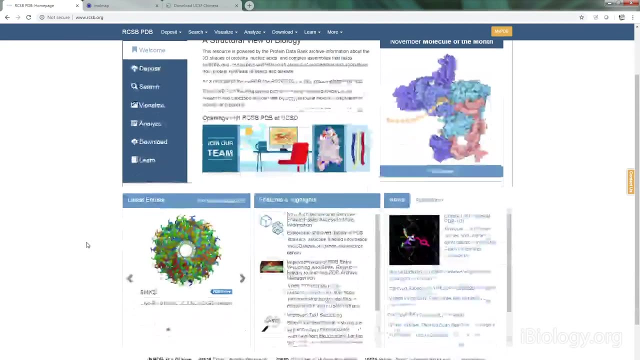 of importing a molecular structure. UCSF Chimera is a. you can just check out the website online and download a version that works for your computer. Then we'll go over to the PDB. So this is a database of molecular structures. 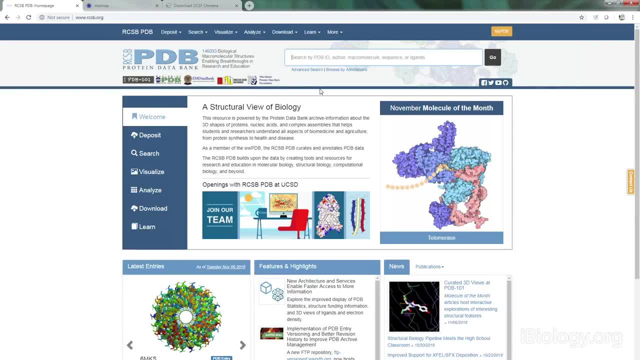 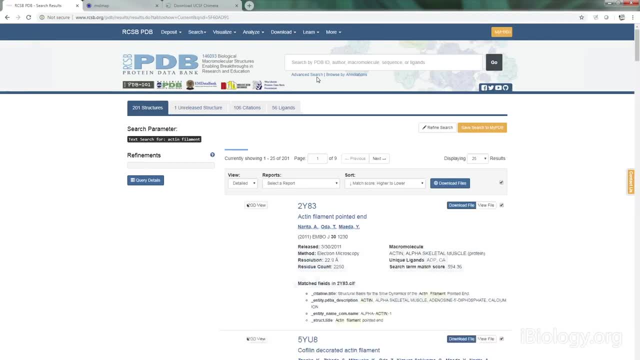 And in this case we're looking for a structure of actin, actin filament that we'll be animating later. So I'll go ahead and do that search And you can see there are a number of bits that we have here. 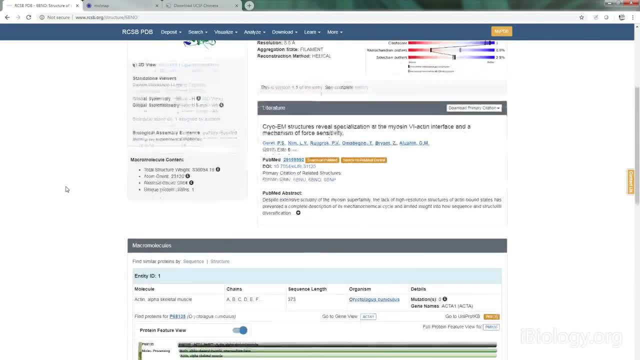 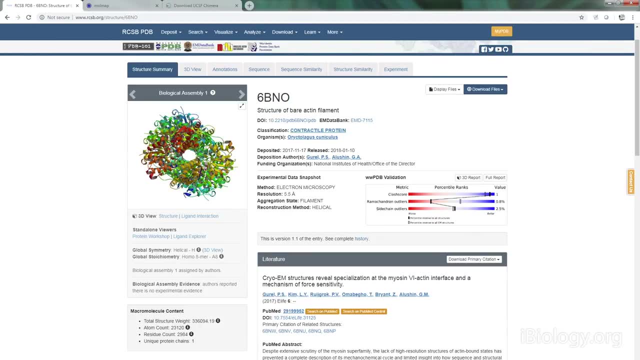 So we can go ahead and select one and take a look at this. So this one is called 6BNO And that is what we're going to put into Chimera. So here's Chimera. So what we're going to do. 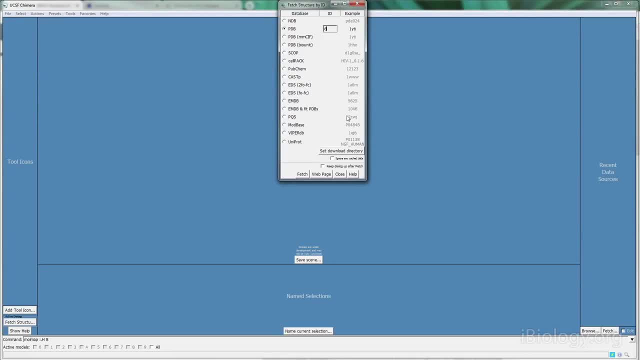 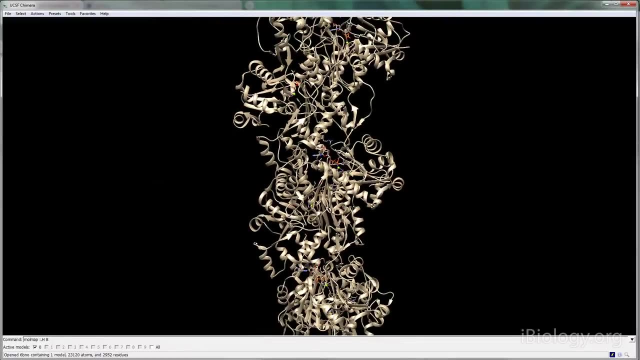 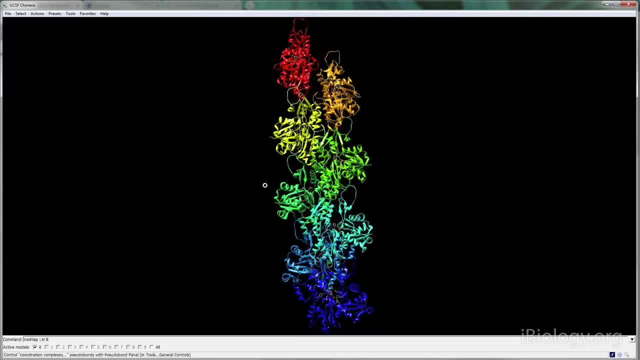 is fetch by ID and put in that that PDB ID here And that'll give us this structure that it just fetched from the web. So we'll go over this using a preset so that the different chains are different colors, So you can see we have. 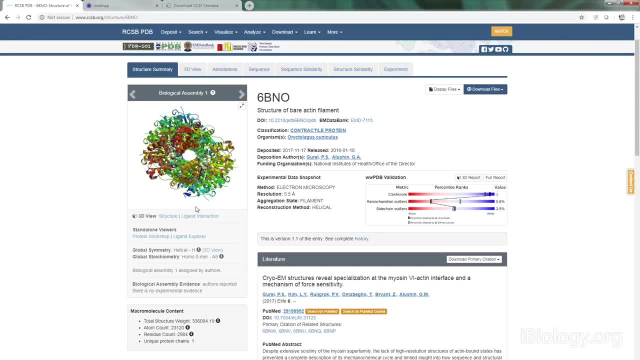 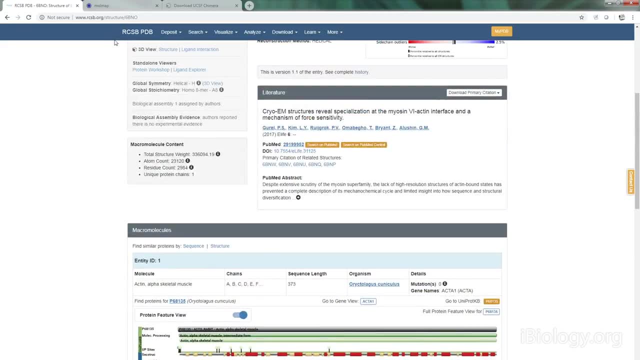 8 different actin monomers here, And those are also listed on the PDB. So you can see chains A through H are all actin monomers, And so what we'll want to do in Chimera is to use a command to create. 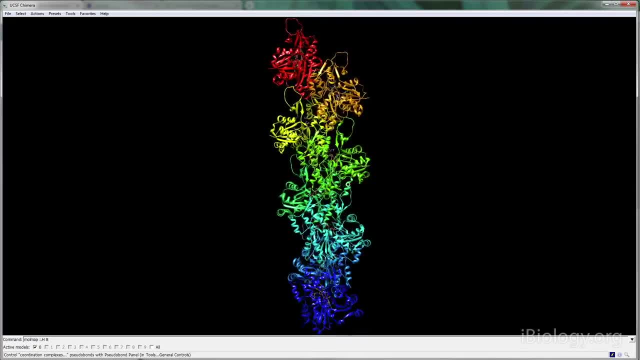 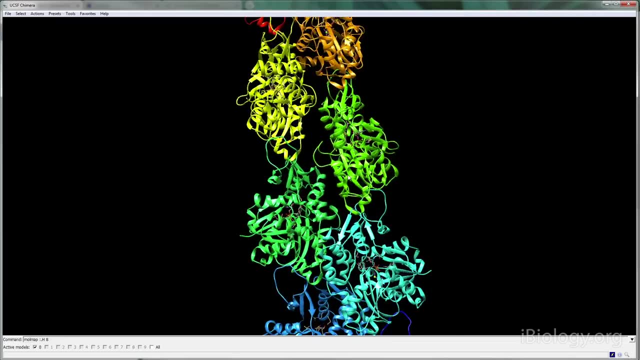 surfaces on this. So these are by default shown as ribbons And typically for molecular animation. you don't really want to support things as ribbons. It's just really kind of a lot of geometry And in general, if you have a lot of molecules. 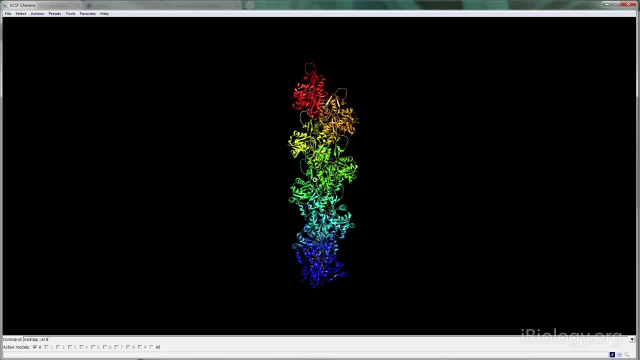 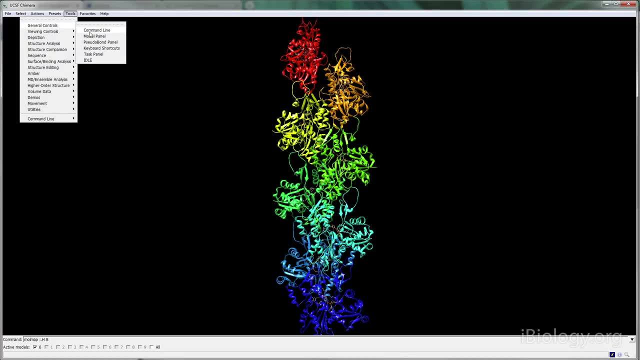 it's a lot easier to visually distinguish them if you use a surface, And so what I use to create surfaces typically is a command called molmap, And so you can find where the command line is by using this command line in the tools And then the command line. 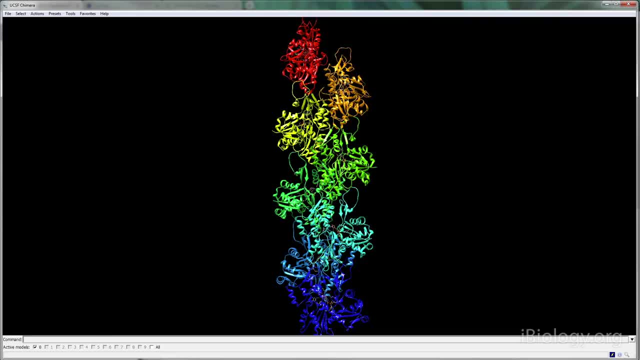 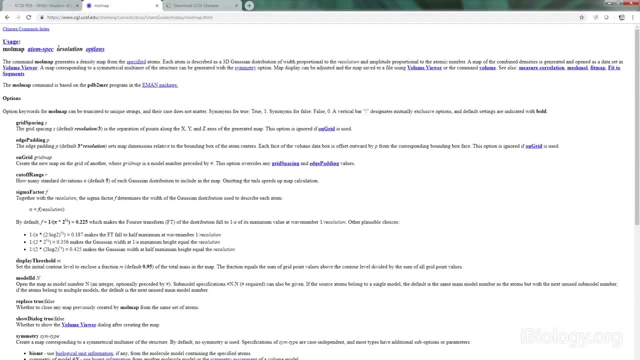 appears down here, And so the molmap command. you can learn more about it using the documentation that's available with Chimera. So, basically, what you have to do is, in the command line, write molmap and then specify a specific atom and name. 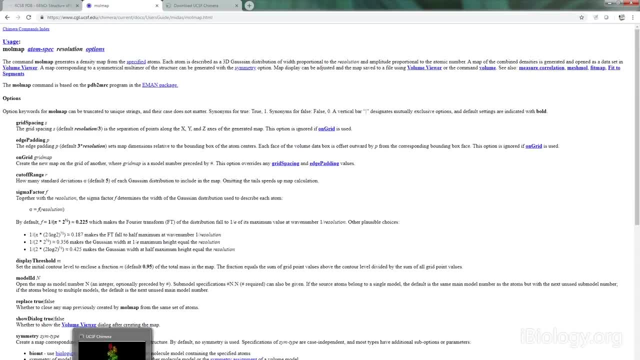 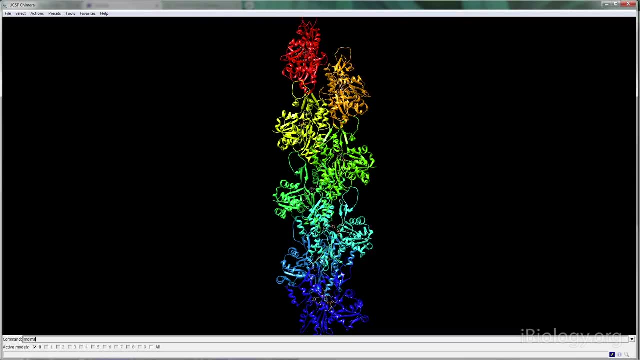 and also include a resolution, a number for the resolution you want to use, And so I'll just show you how that's done. And so, in this case, what we'll do is we'll create a surface for chain A, which is one of the monomers. 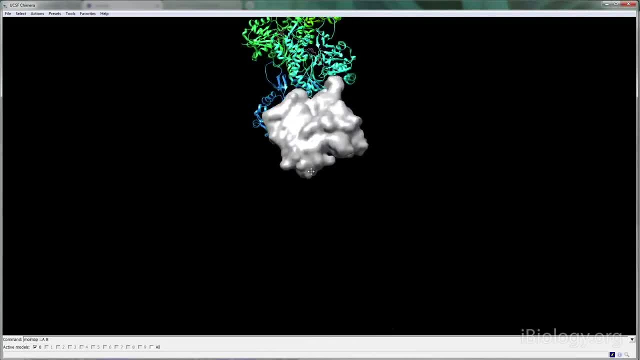 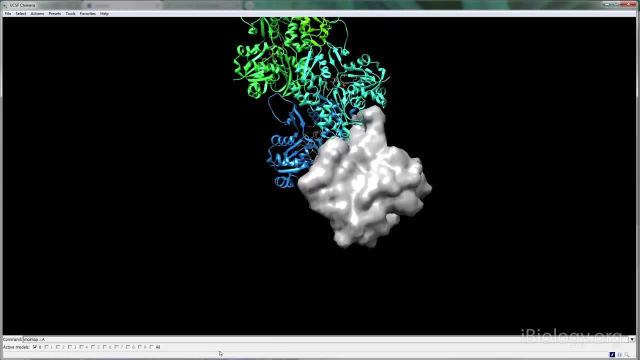 at resolution 8 is a pretty good resolution for a lot of the things I do for the animation we're creating here. So you can see, if we change this number to a lower number you get sort of a bumpier, more detailed surface And a higher number. 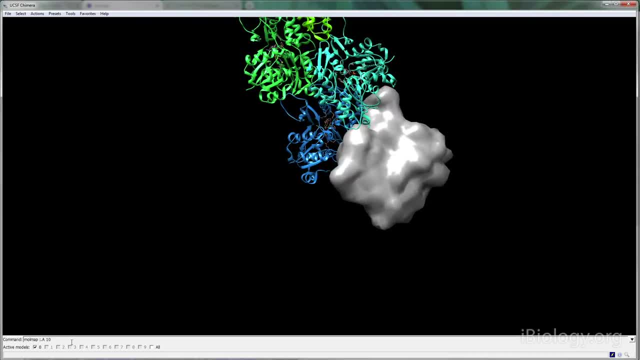 gives you a less detailed kind of smoother surface. So we're just going to go back to 8 and then I'm just going to repeat this command on each of the individual chains so that we have a surface for each of the actin monomers. 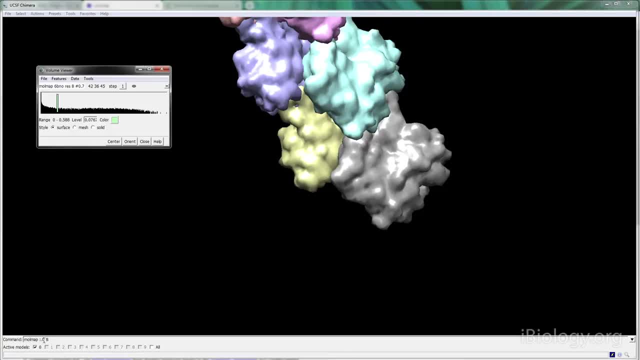 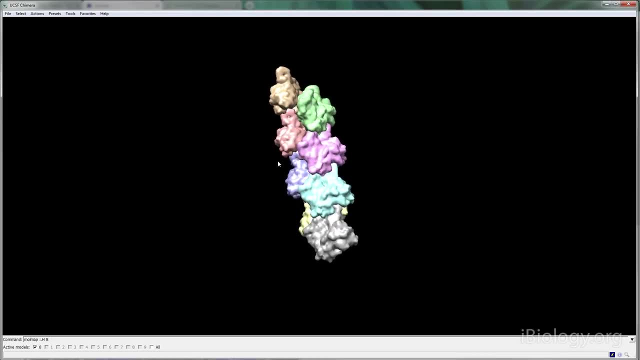 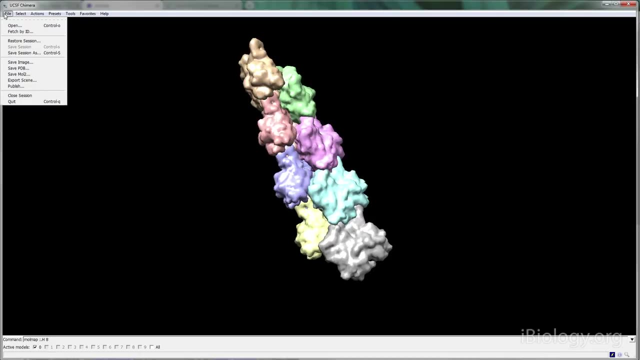 in this filament Through H, And so now you can see that we have the actin filament, this partial actin filament here that has surfaces for each monomer. So now what we want to do is export this as a surface so you can export. 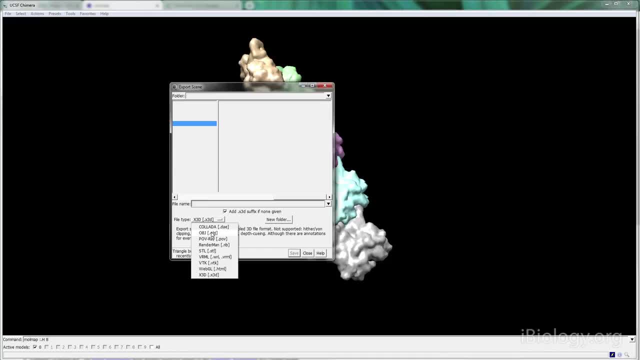 scene And Chimera has options that include things like OBJ, which we can use to directly import into the 3D animation software. So I'm going to call this actin filament and then I'll also include the PDB for reference and save. 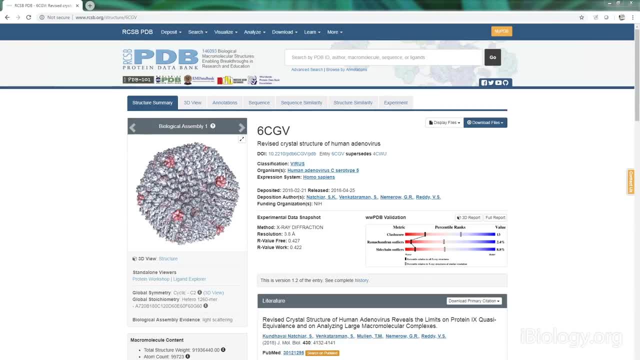 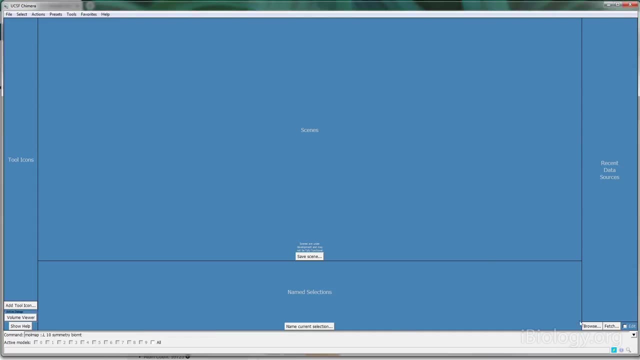 that. So something else you can do using Chimera is to take a look at some larger structures. So in this case I'm taking a look at this human adenovirus structure 6CGV So we can import that into UCSF Chimera. 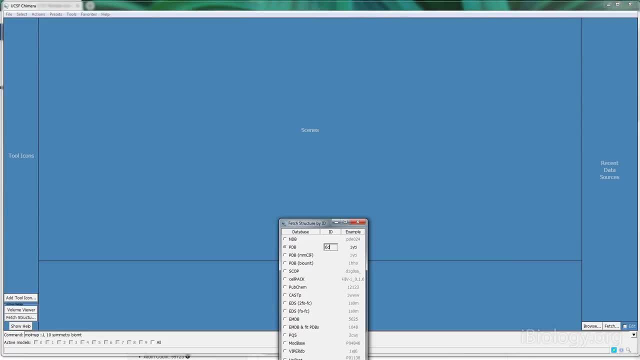 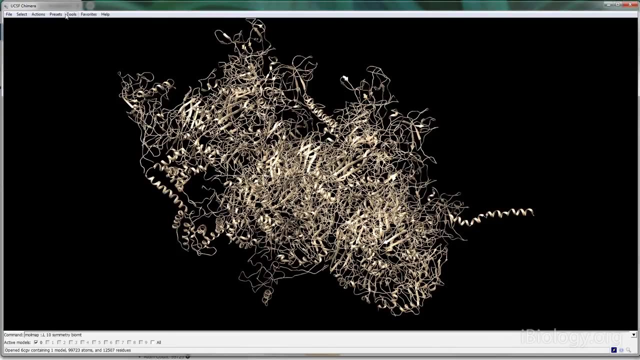 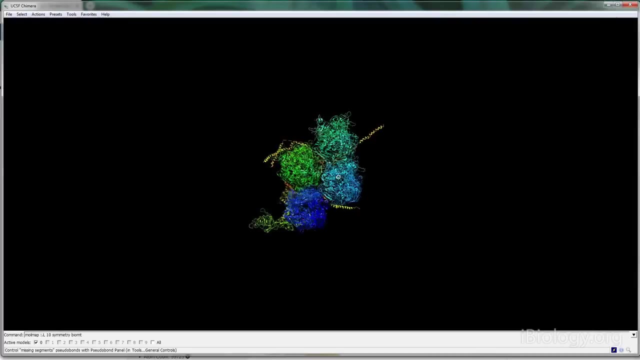 6CGV, and then we can import that into UCSF Chimera 6CGV. And what you might notice is that this is not the entire, the entire capsid that we saw in the structure over here. So one thing to note about. 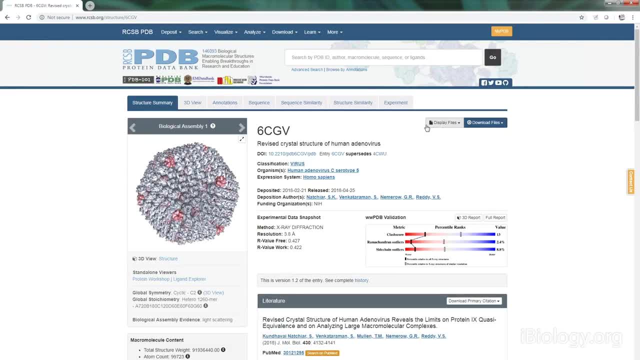 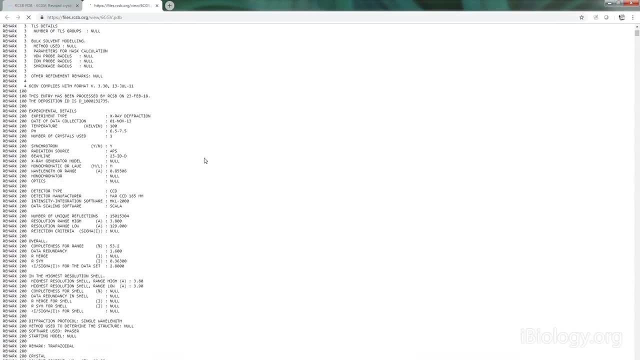 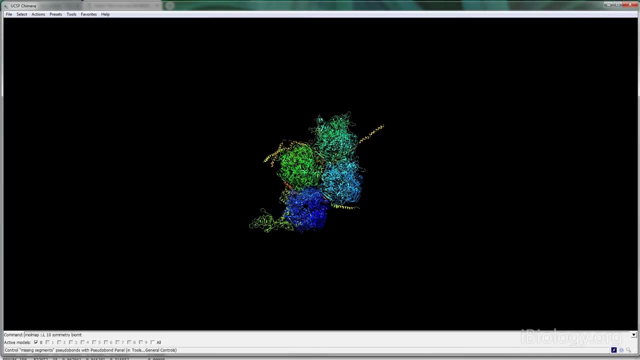 some of these structural files is that you can have some information that's encoded inside the PDB that you might not see immediately in Chimera. So in this case we have some symmetry information about symmetry that's included in the PDB and that we can access in Chimera. 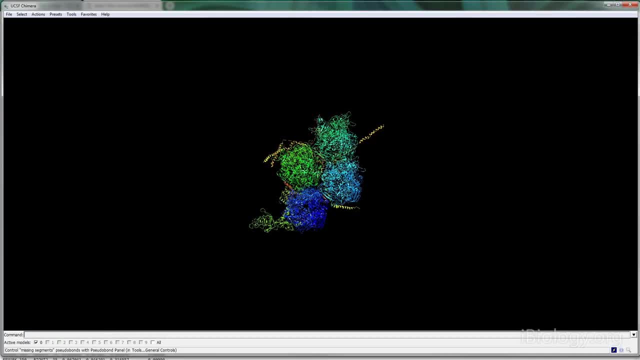 So in this case, what we want to do is use the molmap command, again using chain A- maybe we'll do resolution of 10- and in this case we're going to tell molmap to use the symmetry information that's included in the PDB.